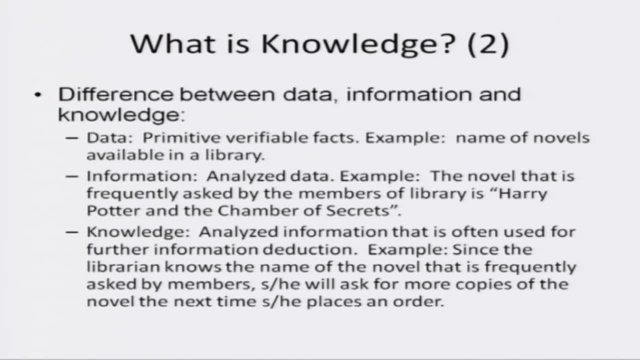 For example, the novel that is frequently asked by members of library is Harry Potter and the Chamber of Secrets. Now, information adds some more value and sense to the data. It enables one to answer some question in a particular context. What is knowledge? Knowledge is further refined. 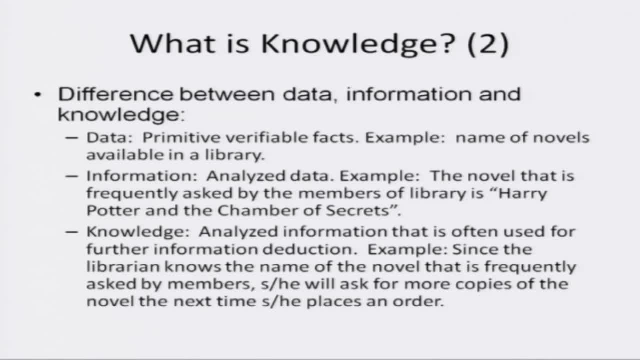 and analyzed information that is often used for further information: deduction, For example. now, continuing the previous example, since the librarian knows the name of the novel that is frequently asked by members, that is, Harry Potter and the Chamber of Secrets, she will ask for more copies of the novel the next time she places an order. 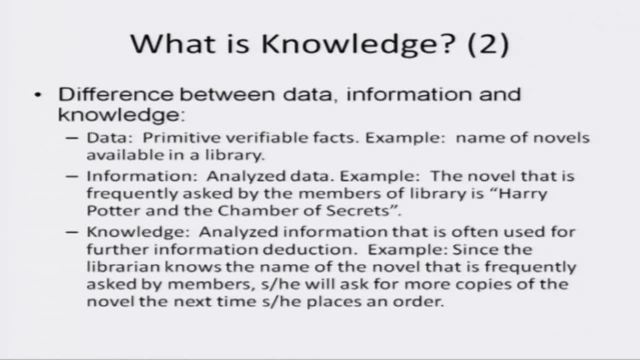 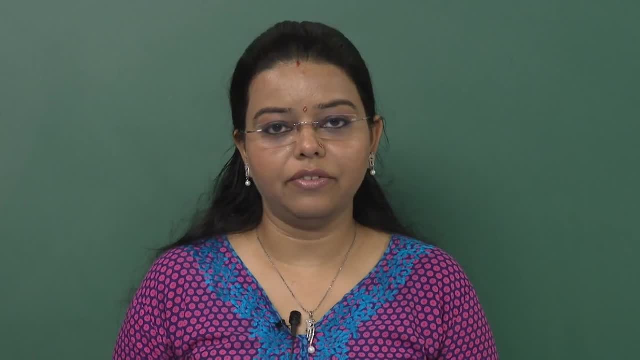 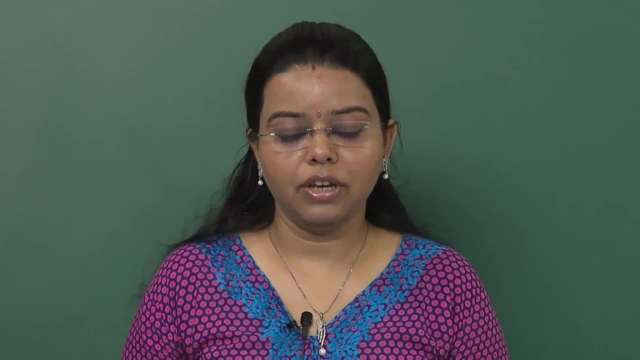 so that all the different requests of the members of the library are fulfilled. Why do we need knowledge representation? We human beings can directly perceive and acquire knowledge in the form of mental images, objects, properties and their relationships. For example, consider a person who has never. 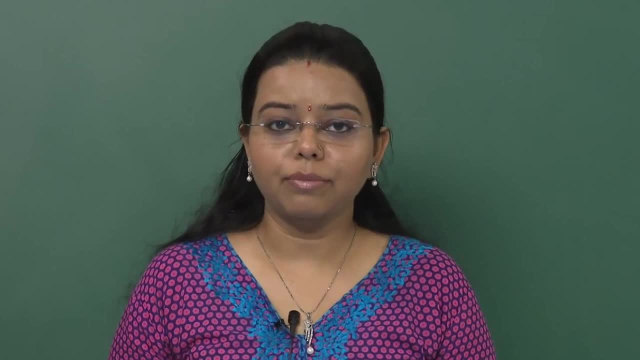 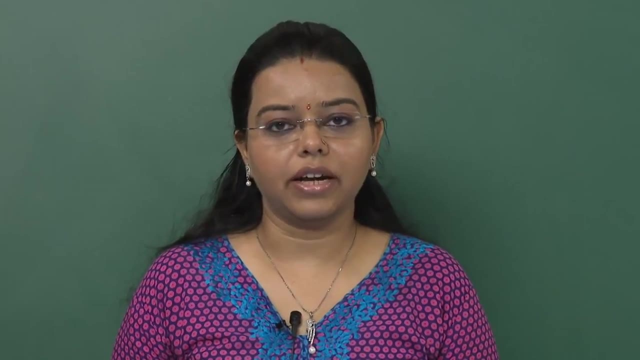 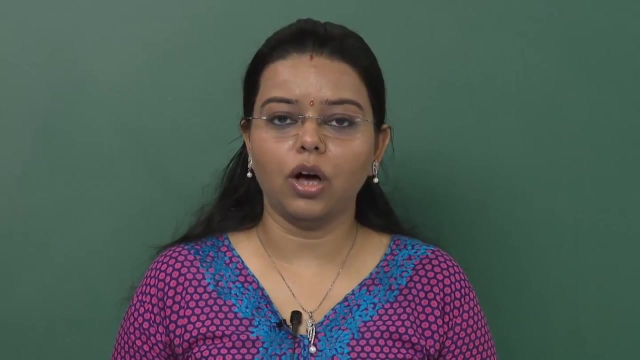 had any experience with a handheld device, say a smartphone, and she happens to take that device into her hand, She plays with it for a while and memorizes her experience of the device, along with its essential features. The person will automatically store all the essential features of the device and retrieve. 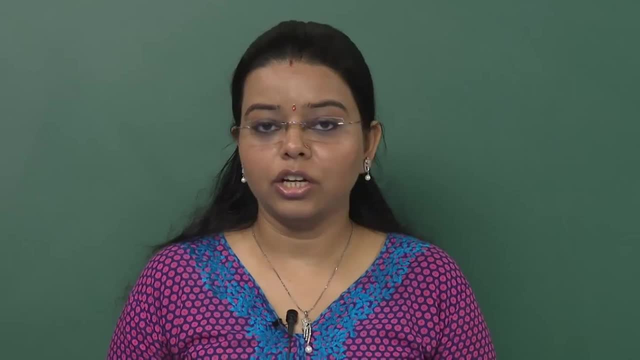 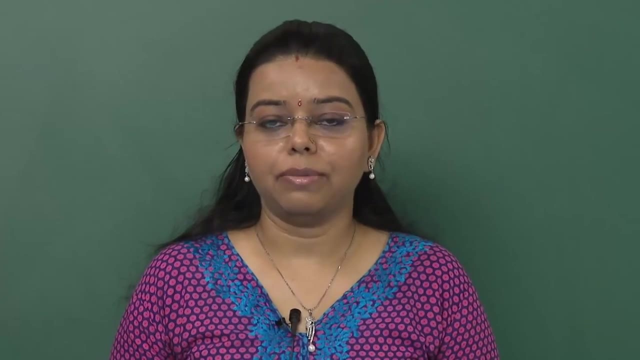 that knowledge the next time she takes that device into her hand. Not only that, if the person has already had an experience with some desktop or a laptop computer, she may very easily get along with the device by automatically reasoning the possible features of the device. 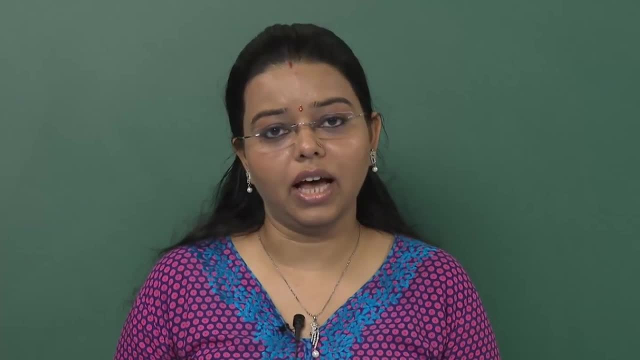 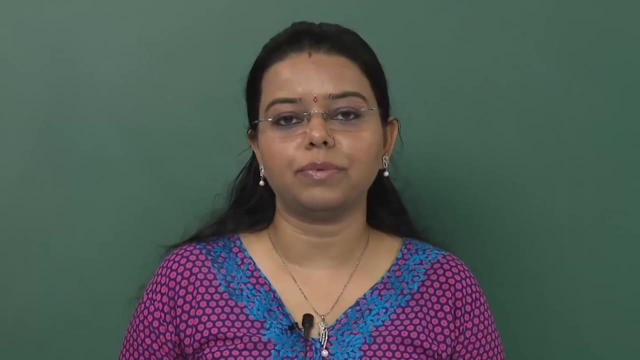 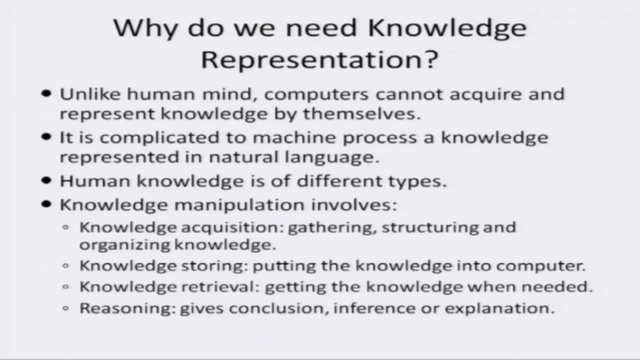 Now this capability is not there with the computers. They rely on human beings to put knowledge into their memory. We therefore have to design some suitable knowledge representation techniques that can represent the knowledge into the computer memory. It is complicated to machine process a knowledge represented in natural language. 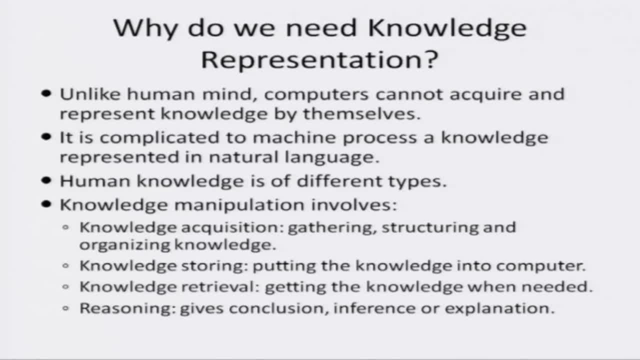 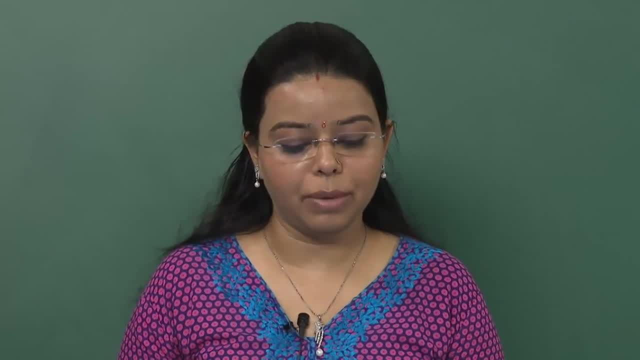 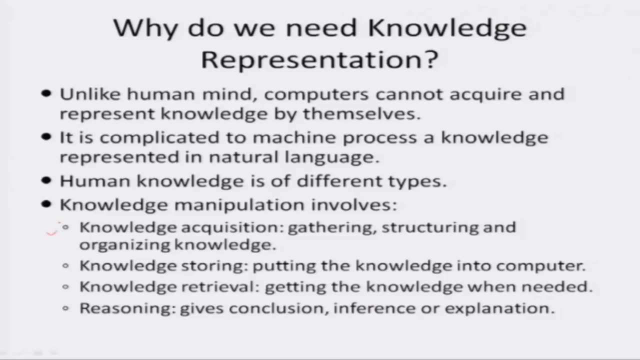 Human language is of different types. Therefore it is essential to suitably design some knowledge representation techniques to efficiently represent the human knowledge into the computer memory. Knowledge manipulation involves these activities. First of all, knowledge acquisition: It is the process of gathering, structuring and organizing knowledge of a particular topic. 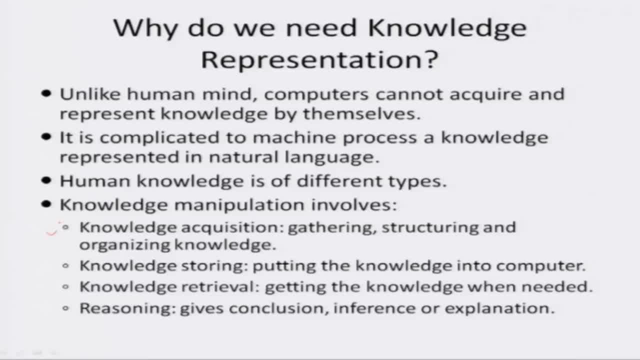 or a domain in order to prepare it to be put into the computer memory. Knowledge storing is the process of putting the knowledge into the computer in a suitably encoded format. Knowledge retrieval is the inverse process of getting the knowledge back whenever it is needed. 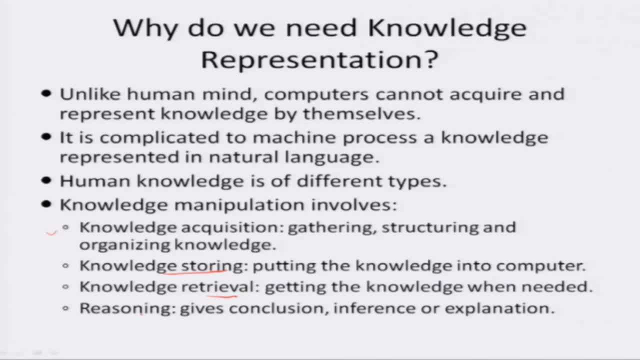 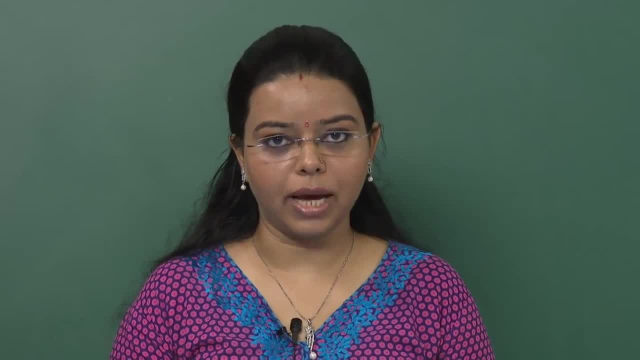 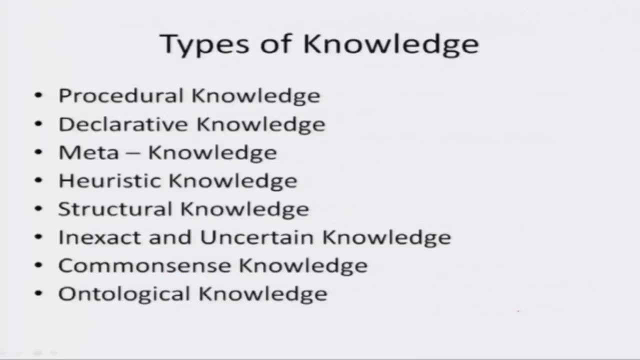 Reasoning. This is the most important part of knowledge representation. It includes deriving new knowledge from the existing knowledge by means of an intelligent program. The newly derived knowledge is known as conclusion, inference or explanation. The different types of human knowledge are: procedural, declarative, metanowledge, heuristic. 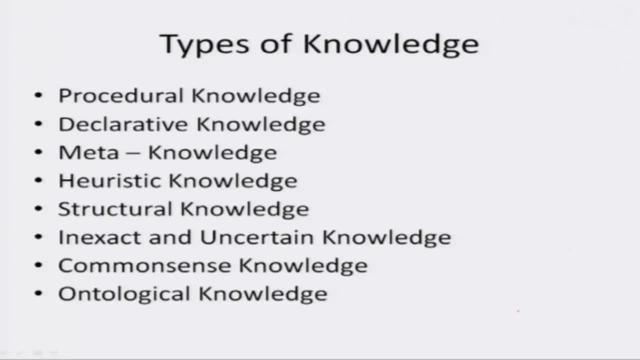 structural, inexact and uncertain knowledge, common sense knowledge and rational knowledge. The most important part of knowledge representation is the process of generating new knowledge from the existing knowledge by means of an intelligent program. It includes intergral knowledge and ontological knowledge. 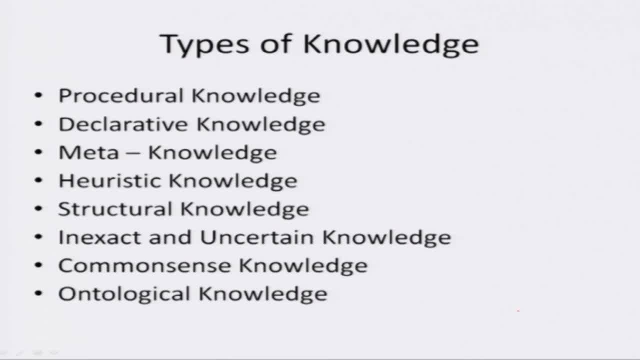 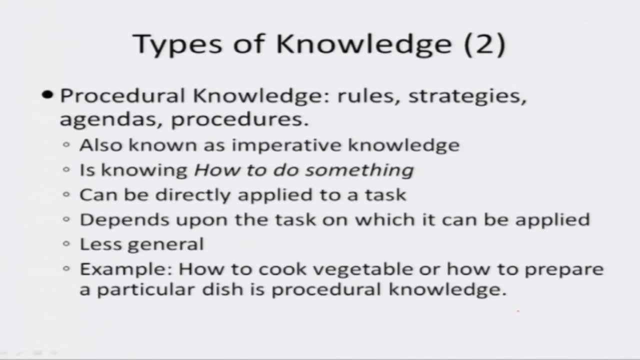 We will be discussing each one of them very briefly. First of all, the procedural knowledge. It includes rules, strategies, agendas and procedures. It is also known as imperative knowledge. It is actually knowing how to do something or a particular task. It can be directly applied to a task. 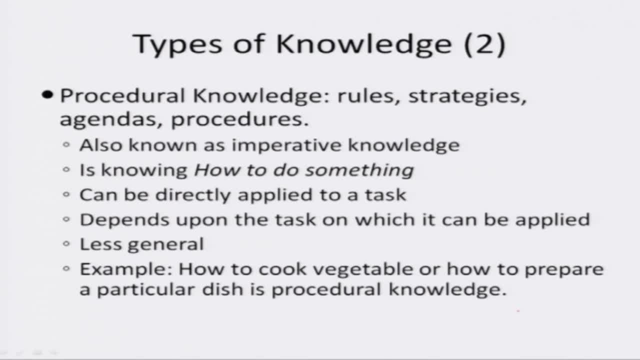 It also depends upon the task on which it can be applied, For example, how to cook vegetable or how to prepare a plate. Then it includes rules, strategies, memoirs, SLAs and procedures. It is also known as imperative knowledge. How to prepare a particular dish is procedural knowledge. 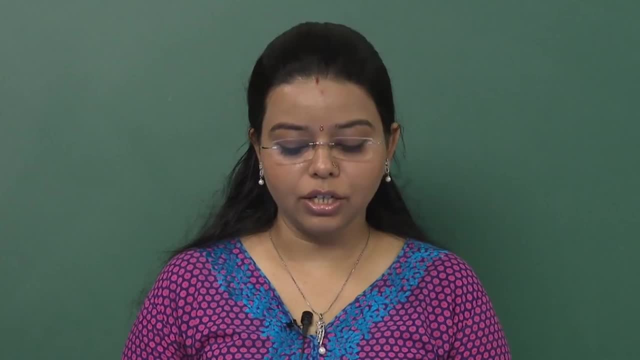 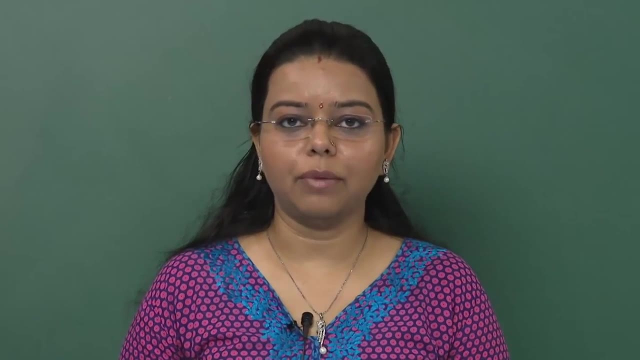 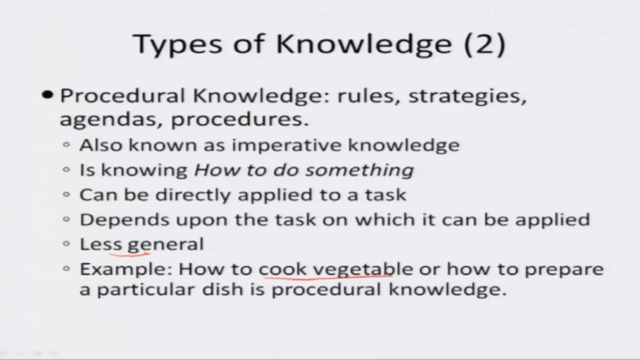 Now, the sequence of steps that are required to be done to cook a vegetable are very much task dependent. They cannot be applied to do some other task, for example bake a cake, for instance. So this knowledge is very much task dependent and hence is less general. 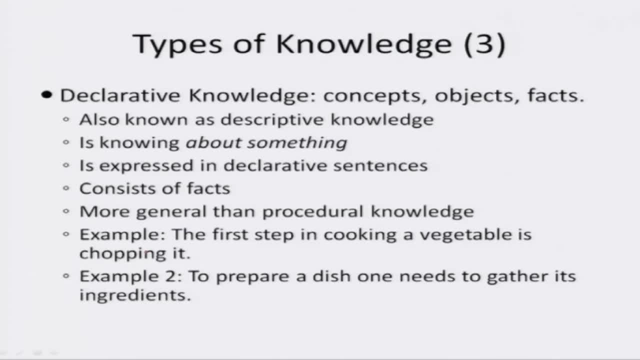 Declarative knowledge. It includes concepts, objects and facts. It is also known as descriptive knowledge. It is knowing about something. It is expressed in declarative sentences and is actually a collection of facts. It is more general than procedural knowledge. For example, the first step in cooking a vegetable is chopping it. 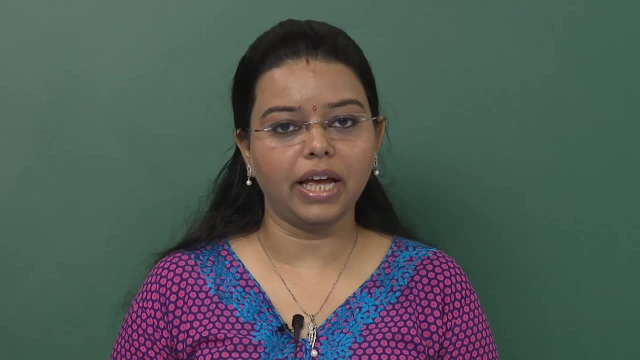 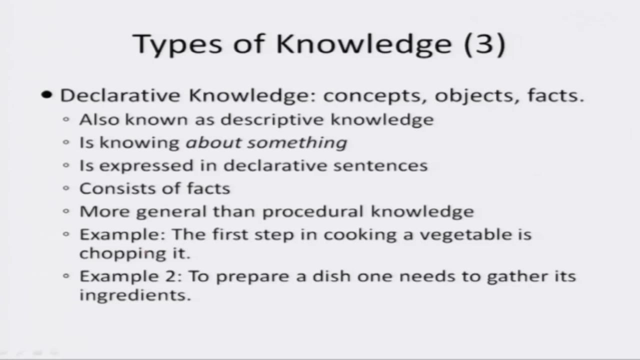 Now, this statement is general enough to be applied to cook any vegetable. Another example is to prepare a dish, one needs to gather its ingredients. Again, this is general enough to prepare any dish, And therefore Declarative knowledge is more general than procedural knowledge. 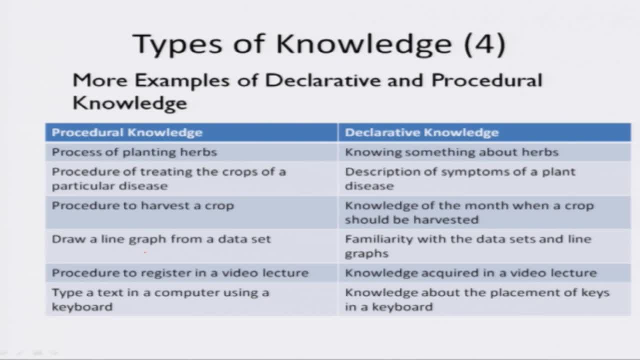 To understand more clearly the difference between declarative and procedural knowledge, let us see some more examples, For example, process of planting herbs. This is a sequence of steps, for example, collecting the different seeds, sowing them into the soil and then watering them appropriately. 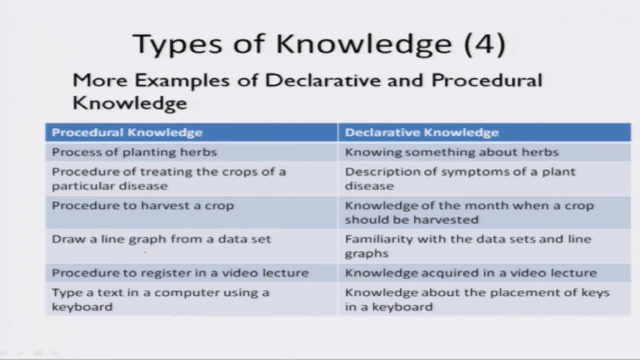 Since it consists of a sequence of actions, this is procedural knowledge. Declarative knowledge is more general than procedural knowledge, But, knowing about herbs, this is a collection of facts and hence is declarative knowledge. Procedure of treating the crops of a particular disease. 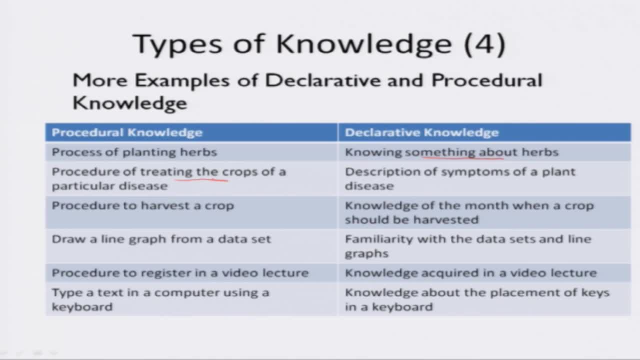 Now, this treatment process is a step-by-step process and hence is procedural knowledge. But description of symptoms of a plant disease is a collection of facts and is therefore declarative knowledge. Procedure to harvest a crop: This is a sequence of actions to be done. 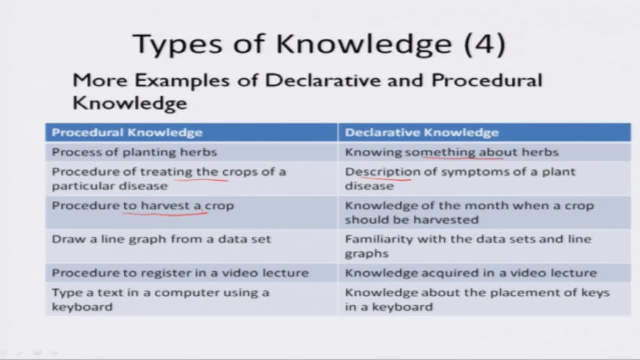 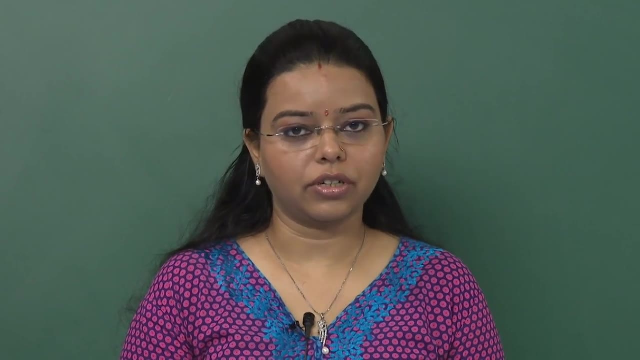 And is therefore procedural knowledge. Knowledge of the month when a crop should be harvested is a fact and is therefore declarative knowledge. Draw a line from a data set. This includes a set of actions. for example, plot the data points onto the graph and then. 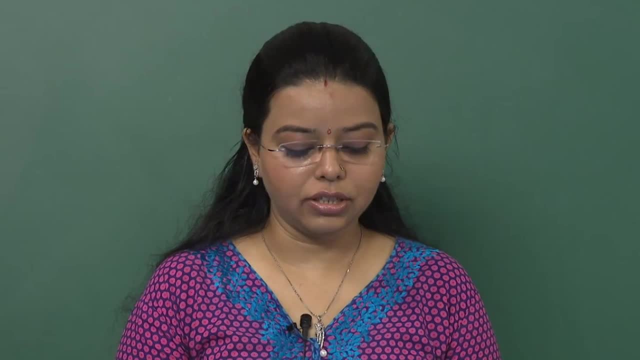 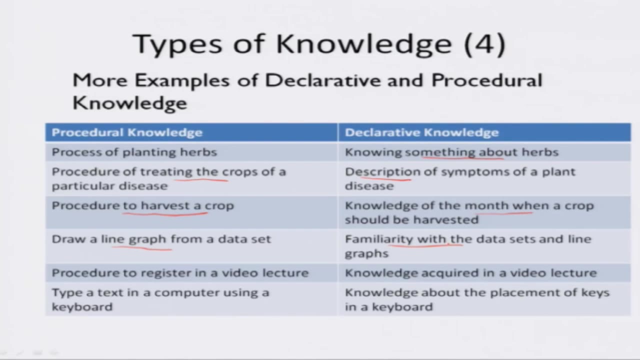 join the points with the line, Since this is a sequence of action. this is procedural knowledge, But familiarity with the data sets and line graphs. this is a collection of facts and hence is declarative knowledge. Procedure to register in a video: This includes sequence of actions to be done to register oneself in a video. lecture and. 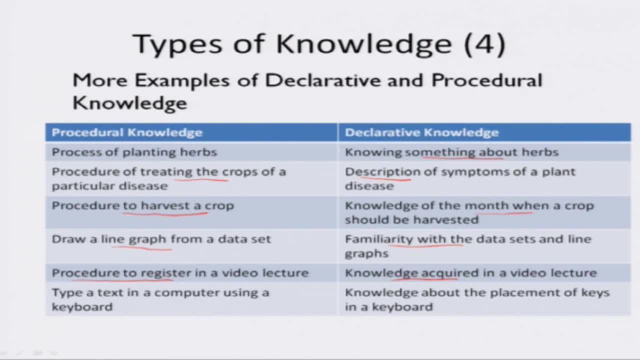 is therefore procedural knowledge. But knowledge acquired in a video lecture is a collection of facts and is therefore declarative knowledge. Type a text in a computer using keyboard involves a sequence of actions of typing into the character, into the keyboard and is therefore procedural knowledge. 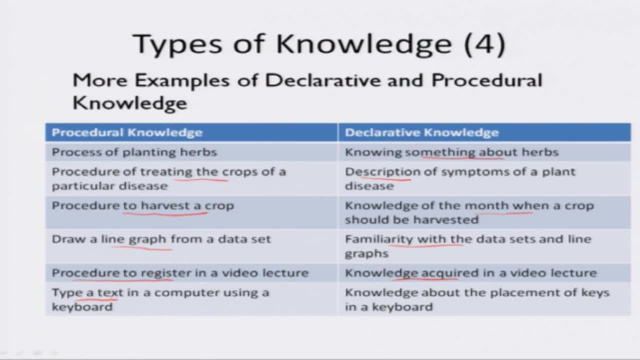 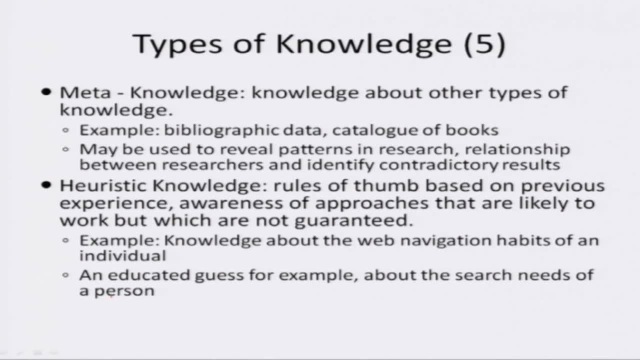 But knowledge about the placement of keys in a keyboard is declarative knowledge. Now meta-knowledge, It is knowledge about other types of knowledge. It establishes relationship between different pieces of knowledge and also enables one to use that knowledge, For example, bibliographic data, catalog of books. 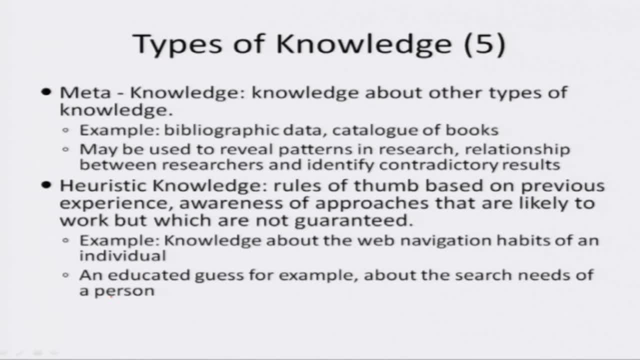 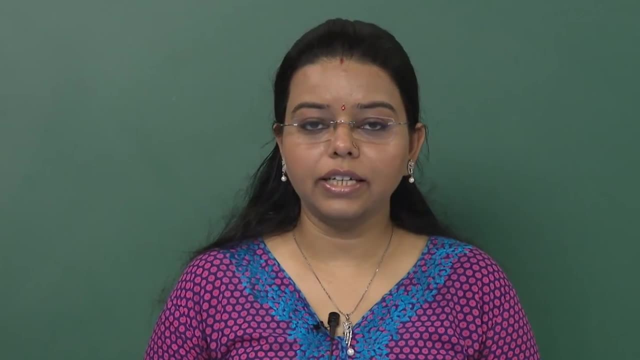 Now the relationship established in bibliographic data can be used to reveal patterns in research relationship between researchers and also to establish the relationship between the data. It can also identify contradictory results in researchers. Heuristic knowledge involves rules of thumb or first principles that guide the problem. 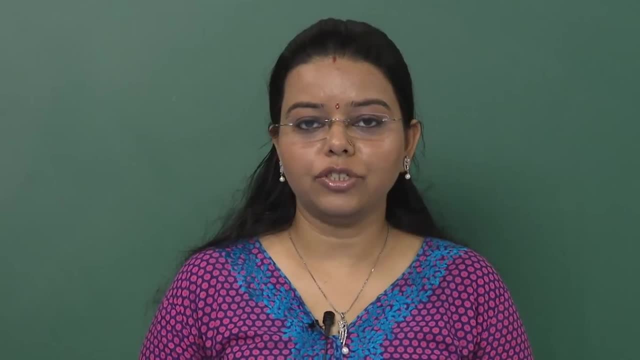 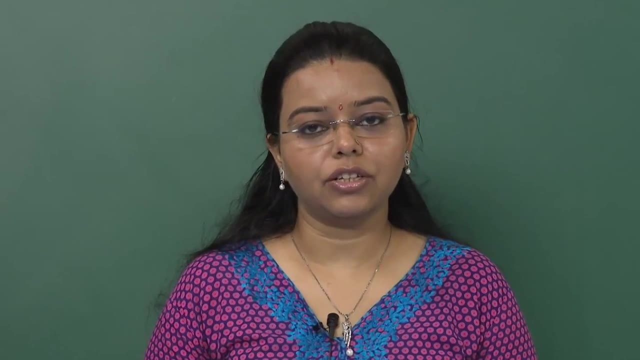 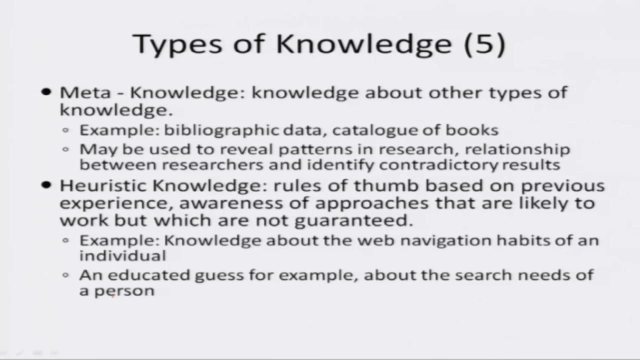 solving process based on previous experience, individual intuition and skills and deep understanding of the problem domain. However, the problem solving based on heuristic knowledge is not guaranteed to be successful. For example, knowledge about the web navigation habits of an individual, An educated guess about the search needs of a person. 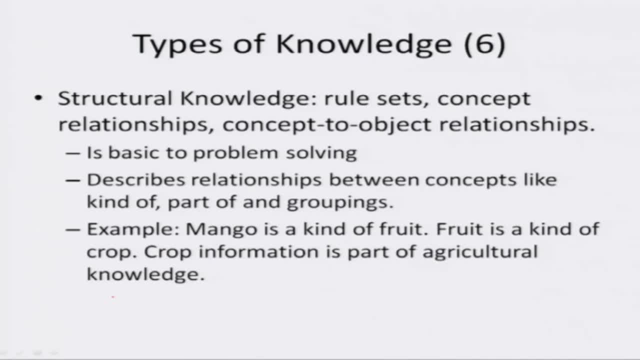 Structural knowledge. It includes rule, sets concept relationships, concept to object relationships. It is basic to problem solving and describes relationships between concepts like kind of part of and other relationships that may enable one to group the concepts. For example, mango is a kind of fruit. 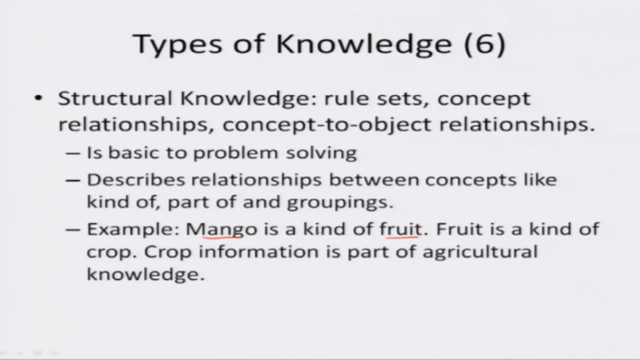 Here, mango and fruit are concepts and kind of is a relationship. It is not a rule of thumb or first principles that can be used to define a person. It is a rule of thumb concept to object relationships. It is a rule of thumb concept to object relationships. 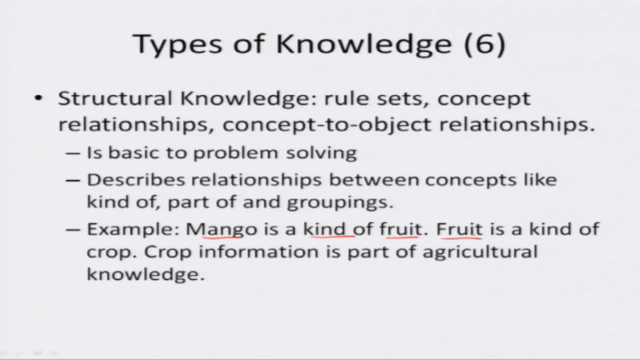 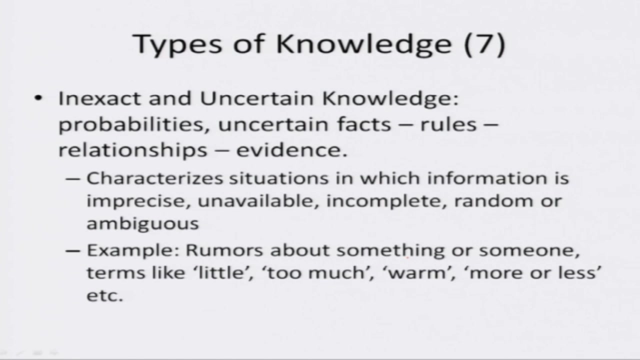 relationship. Fruit is a kind of crop. Here fruit and crop are concepts and kind of is a relationship. Crop information is part of agricultural knowledge. Here, crop information and agricultural knowledge are concepts and part of is a relationship- Inexact and uncertain knowledge. It includes probabilities, uncertain facts, rules, relationships. 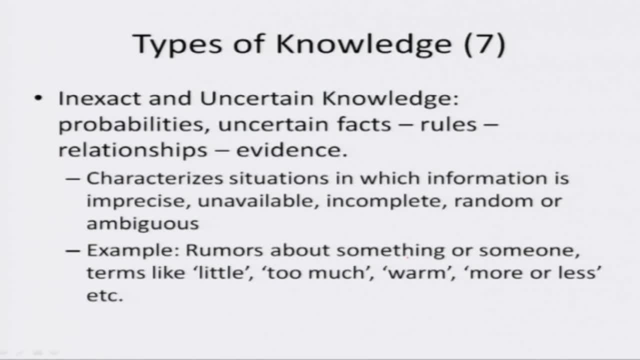 and evidence. It characterizes situations in which information is imprecise, unavailable, incomplete, random or ambiguous, For example rumors about something or someone, Terms like little too much warm, more or less, etc. For example, I may say that this glass of 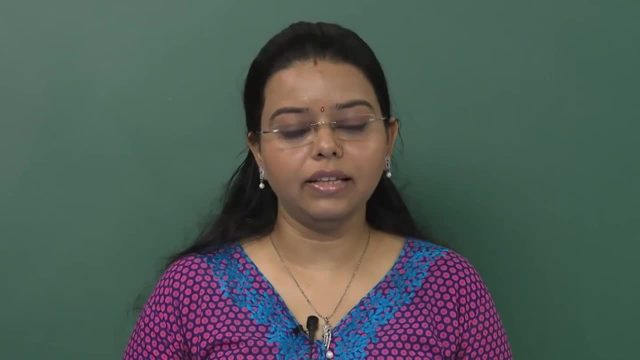 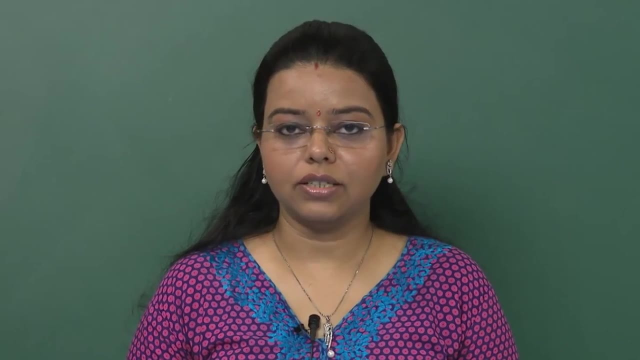 milk is a little hot. This statement does not tell anything about the temperature of the glass of milk. I may say that this room is more or less spacious. It does not give any information about the dimensions of the room. Also, if I say that,